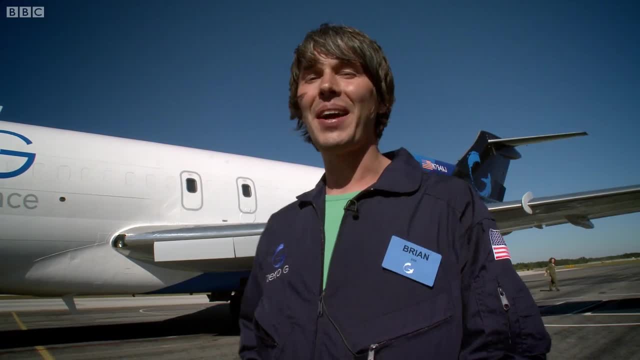 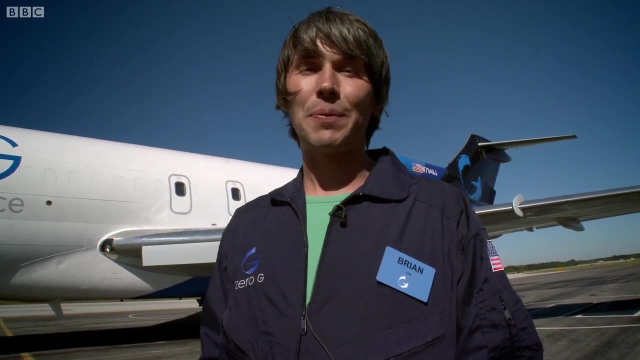 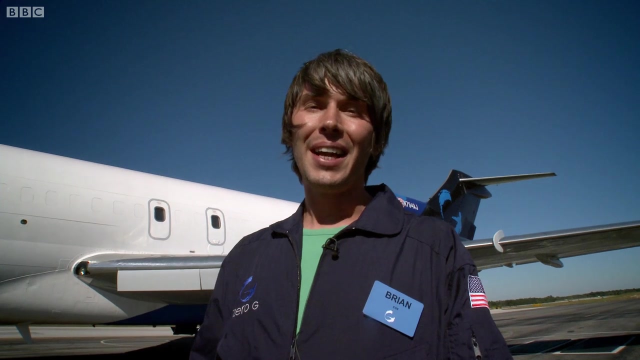 Now, if I was to ask you how do you know that there's gravity around here, then you might say: well, it's obvious. You know, I can just do an experiment, I can drop something. Well, yes, But actually gravity is a little bit more subtle than that. But to really 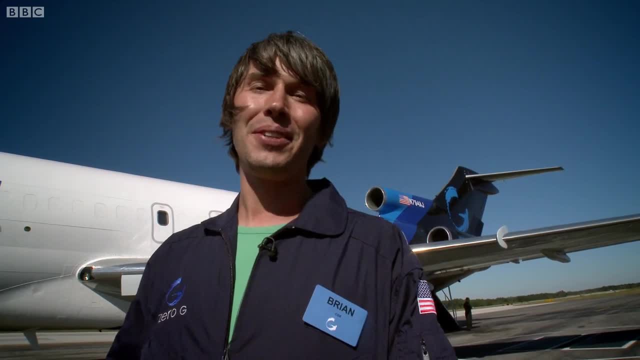 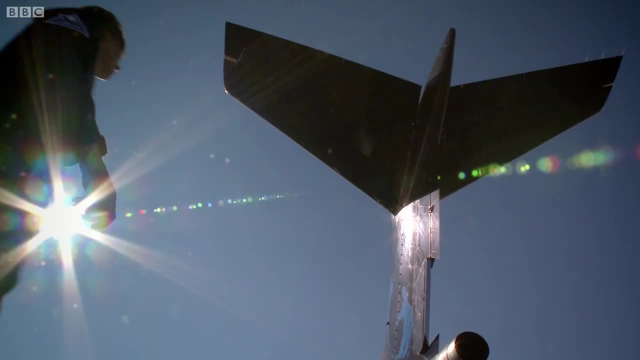 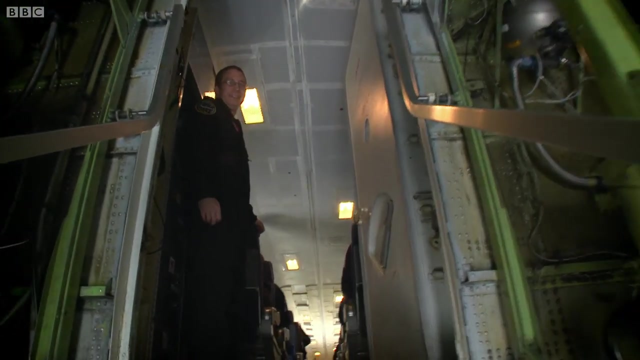 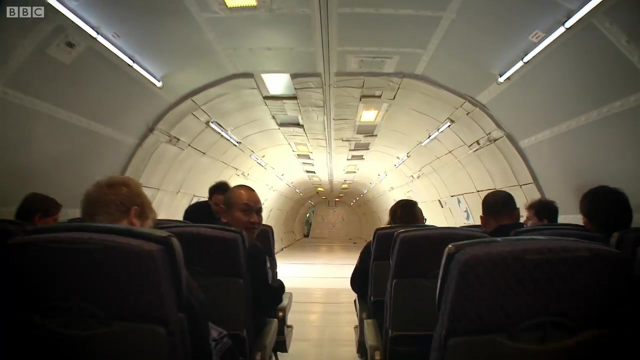 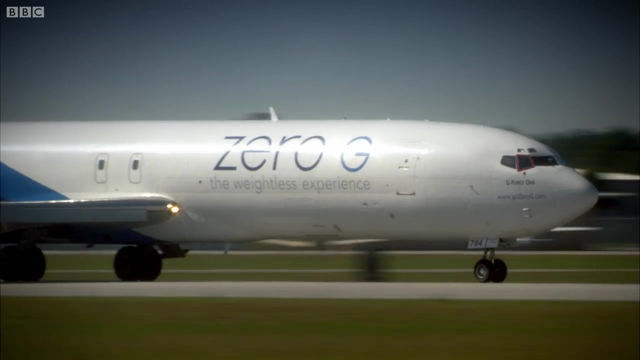 experience it. to understand it, you have to do something pretty extreme, And this plane has been modified to help me do it. Thanks to its flight plan, it's known as the Vomit Comet. Once we've climbed to 15,000 meters, this plane is ready to go. 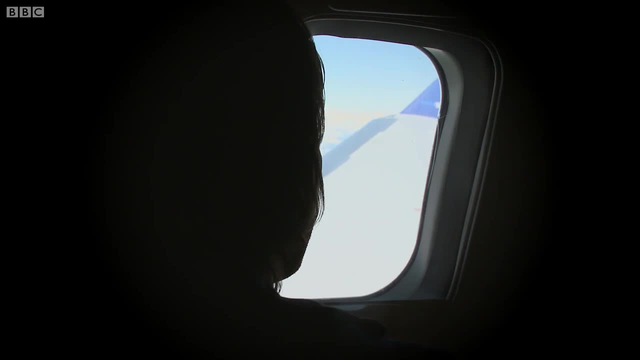 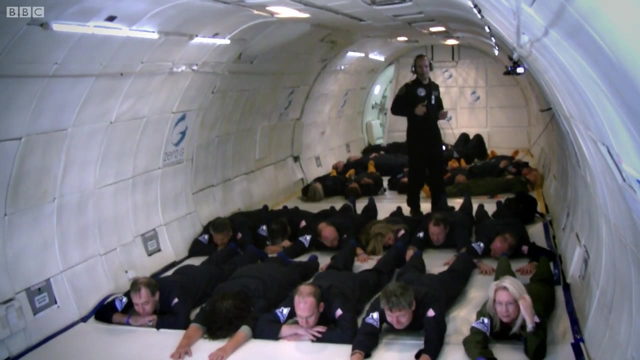 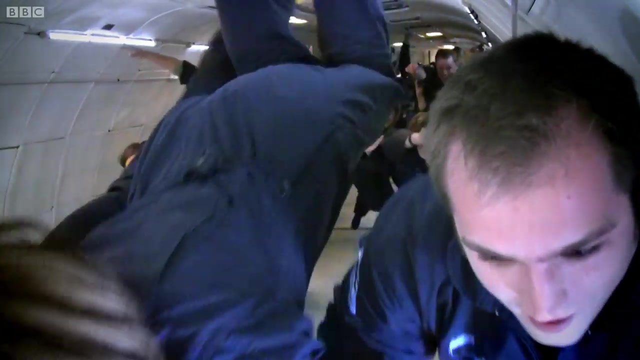 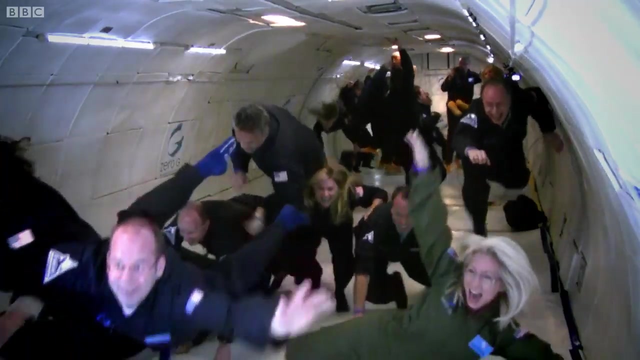 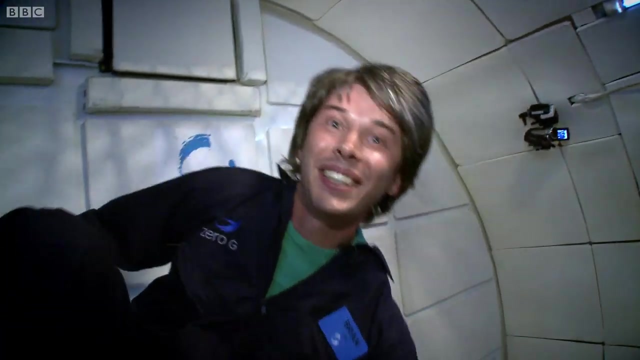 This plane is something no ordinary flight would do. Its engines are throttled back and the jet falls to earth, And then something quite amazing happens. I'm now plummeting towards the ground Just like someone's cut the cable and the lift. 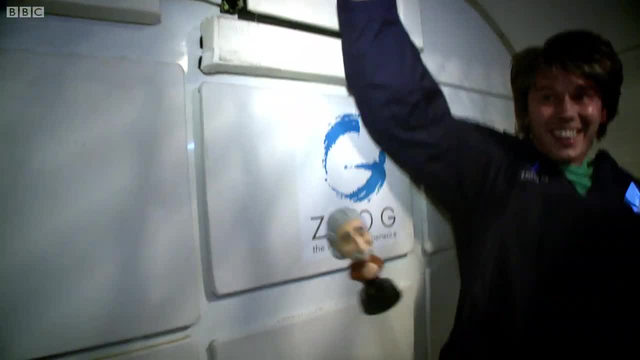 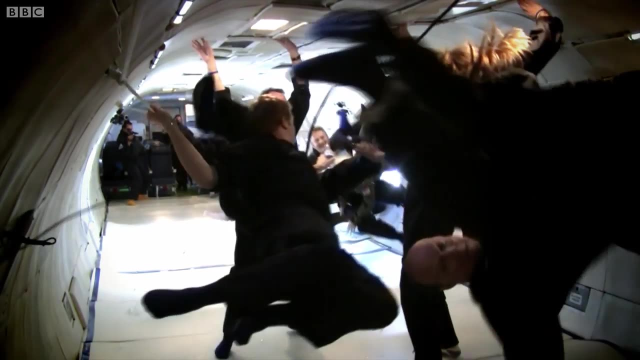 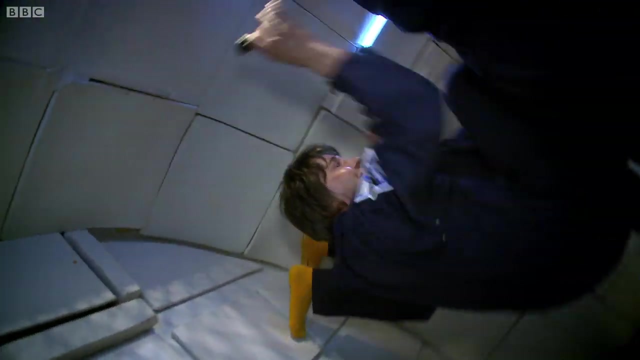 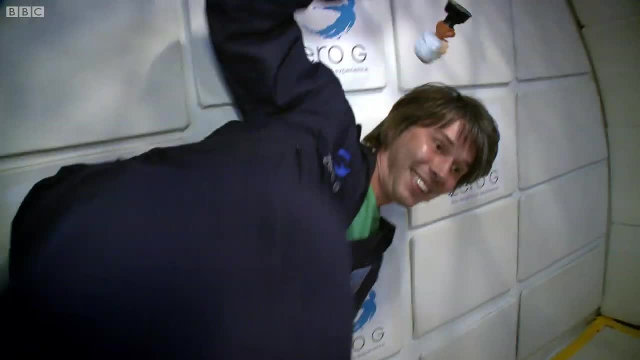 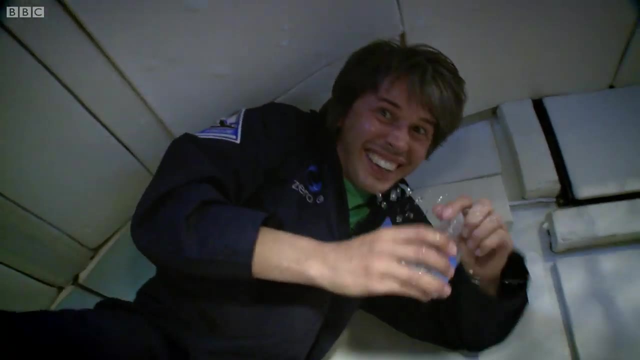 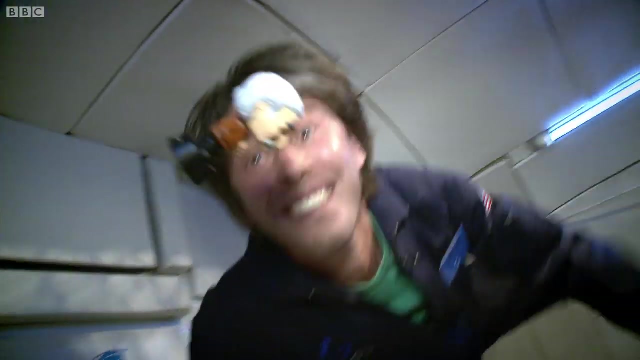